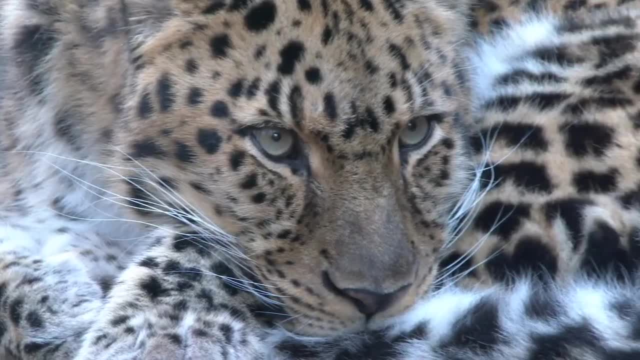 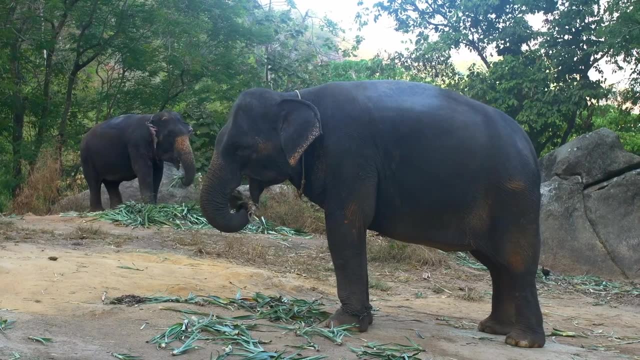 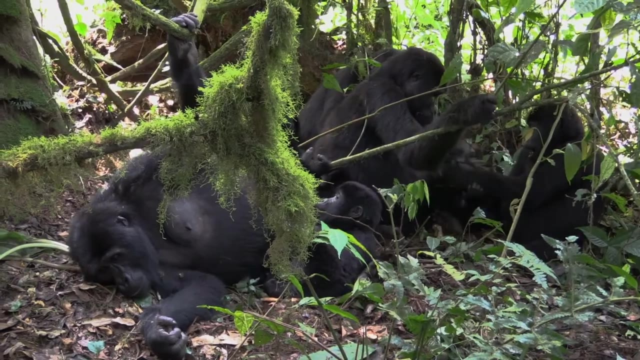 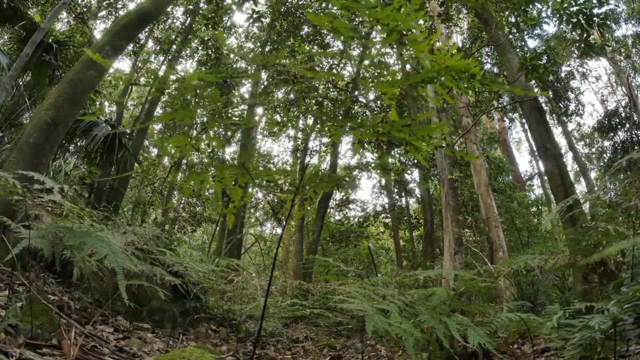 Down here you'll find large mammals like jaguars, tapirs and anteaters. Depending on where the rainforest is, you can also find elephants and gorillas on the rainforest floor. Ferns, mosses, fallen leaves and logs scatter the forest floor. Amongst them, you'll find 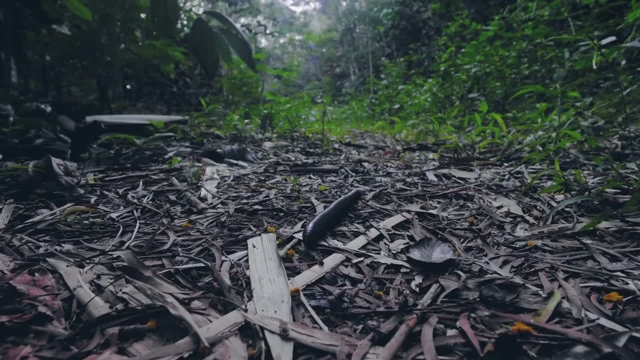 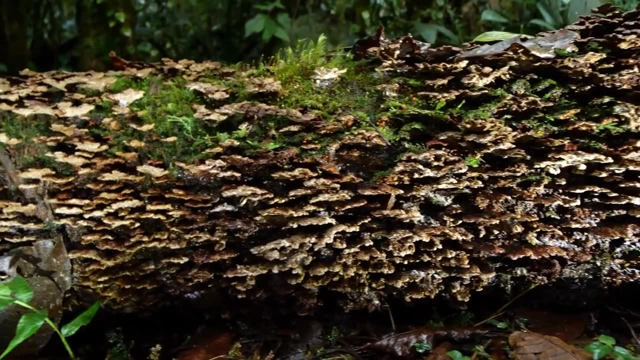 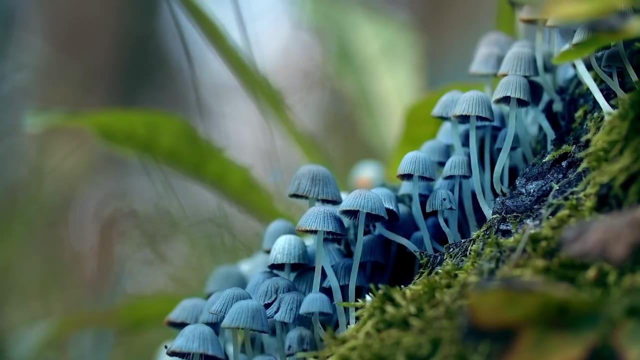 leeches, spiders, centipedes and millipedes and more insects that you can poke a stick at. An important component of the rainforest floor are fungi. These decomposers are constantly breaking down the remains of dead plants and animals. 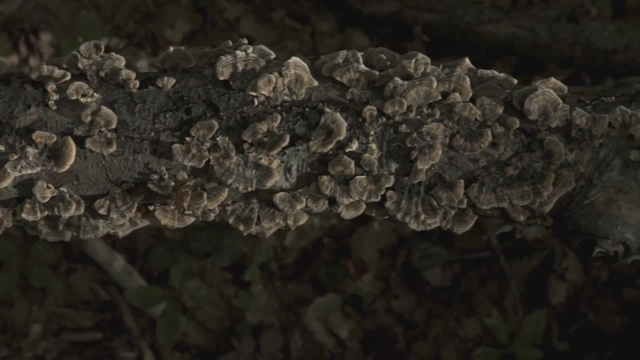 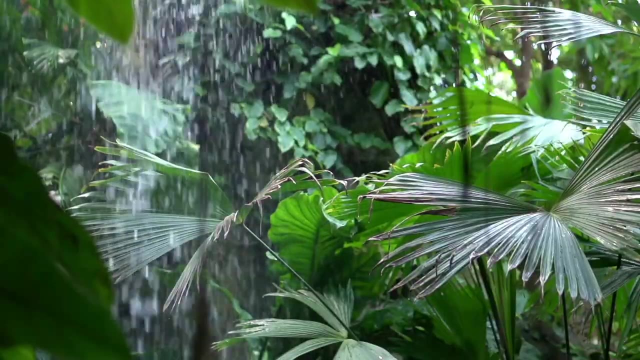 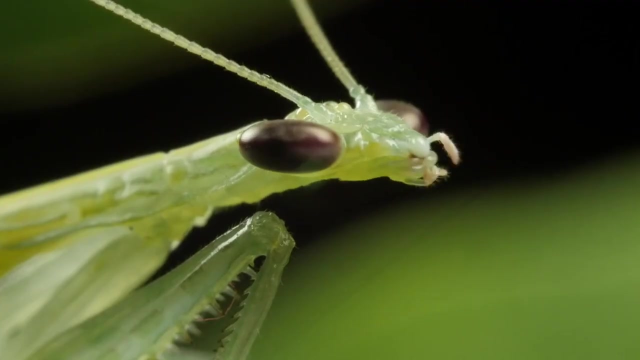 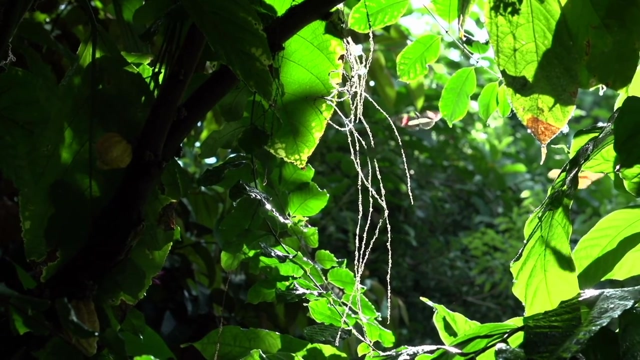 recycling the nutrients back into the soil. As we head off the forest floor, we reach the understory. Here we're talking about snakes, tree frogs, lizards, spiders, praying mantises and leaf insects. The broad leaf plants branch out trying to soak up whatever sunlight they can. 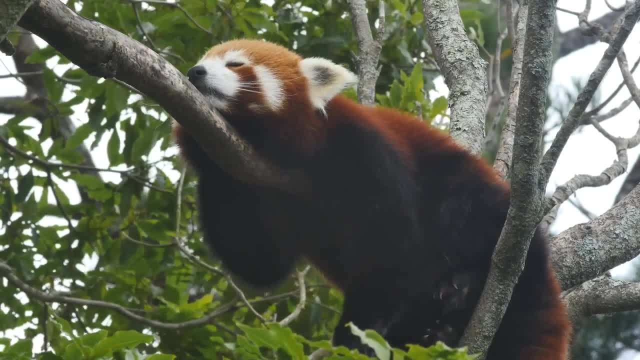 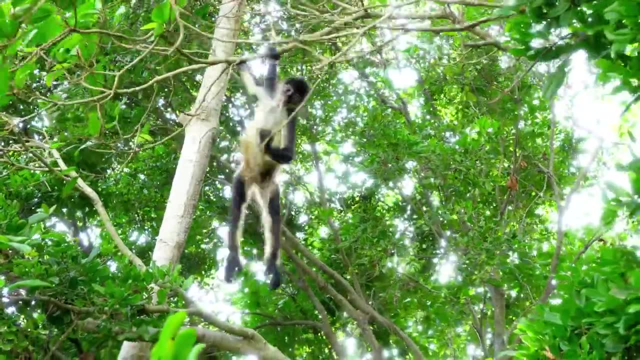 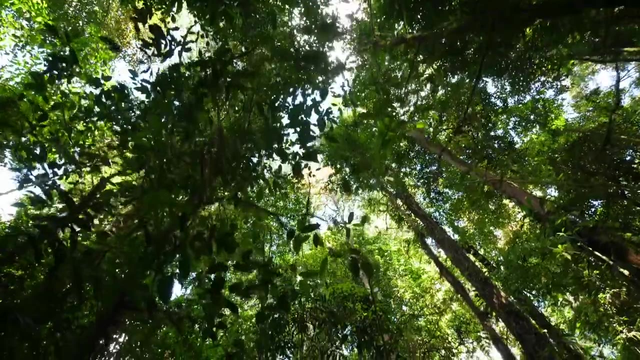 You'll also spot some furry friends like pandas, deer, lynx and squirrels. As we break through the understory, we reach the canopy, A thick layer of overlapping branches and leaves that block about 90% of sunlight from reaching the lower levels. 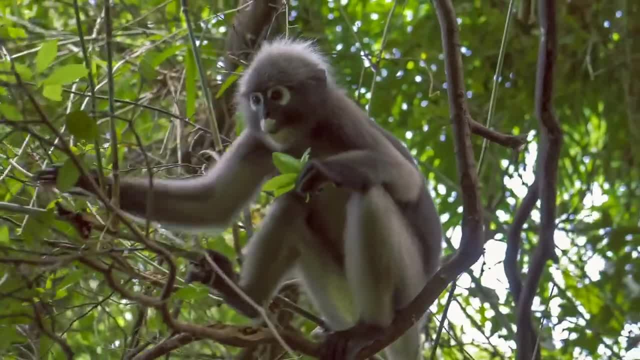 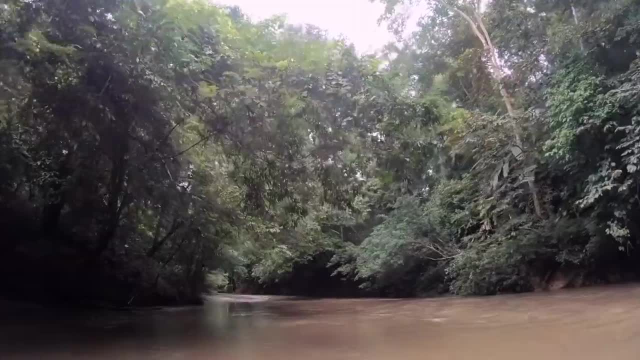 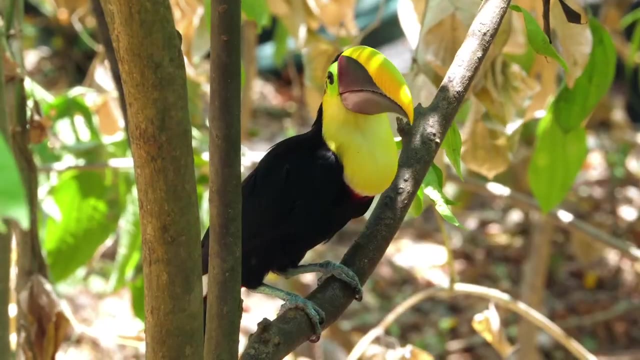 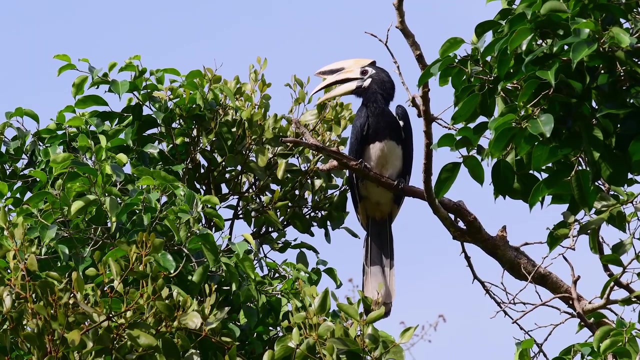 It's here that life flourishes. There's thousands of different types of trees, with their branches intertwined and often tied closely together by a network of creepers and vines. Birds and mammals are common canopy dwellers. There's toucans, macaws and hornbills. 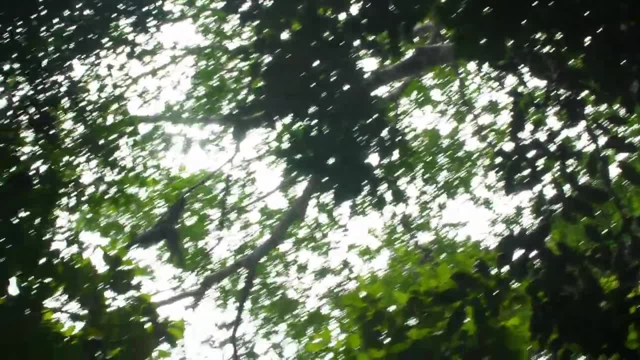 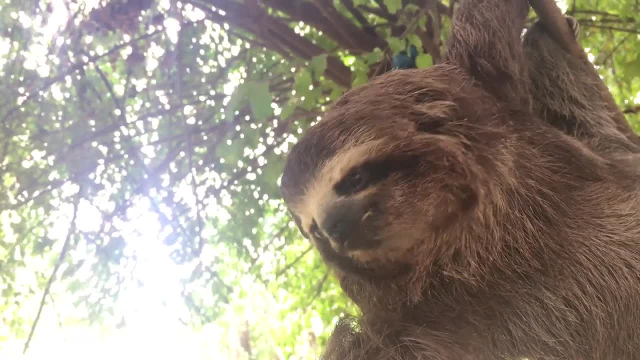 Energetic spider monkeys swing effortlessly through the canopy. They can be found all over the forest. They can feel the heat of the rain, while the ever lazy sloth is happy just chilling out and sleeping. The uppermost layer of a rainforest is the emergent layer.